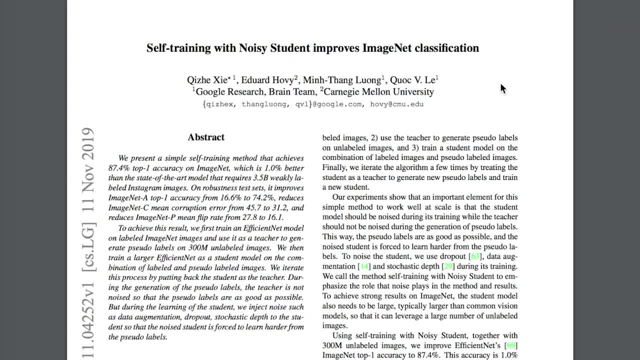 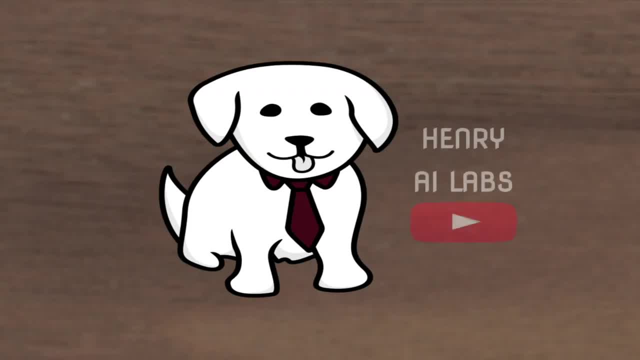 to achieve the state-of-the-art result and they'll also make a compelling case for the integration of noise through dropout stochastic depth and data augmentation to improve knowledge distillation. This video will present the paper. Self-Training with Noisy Student Improves ImageNet. 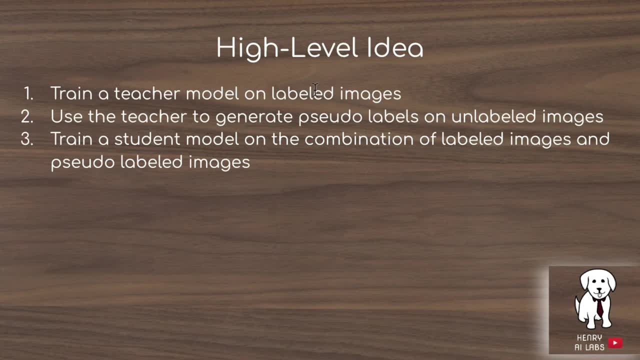 Classification. The high-level idea of the algorithm is to train a teacher-student on labeled images, use that teacher-student to generate pseudo-labels on unlabeled images and then train a student model on the combination of labeled images and pseudo-labeled images. So in this case, 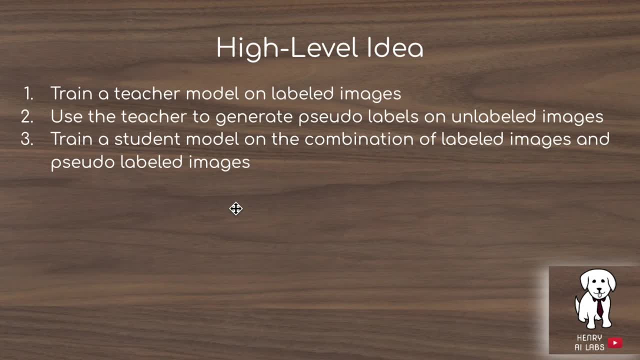 you start with the teacher-student to generate pseudo-labels on unlabeled images and then train the teacher model, say the EfficientNet B7 architecture, and you train it on the ImageNet labeled dataset. Then you use that trained model to generate pseudo-labels or what it predicts. the 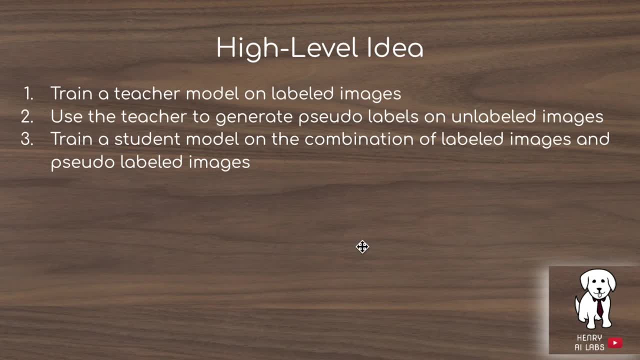 labels might be on unlabeled images, in this case the JFT 300 million dataset. Then you have a student model that is predicting the combination of the ImageNet dataset and the pseudo-labels from the teacher on that JFT dataset. Knowledge distillation is typically a technique used for 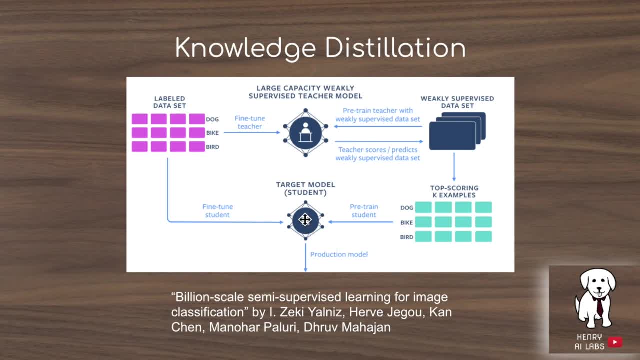 model compression to have a student network that usually has lower capacity for the sake of memory efficiency or faster latency time. So if you have a student network that has a lower capacity for memory efficiency or faster latency time, So if you have a student network that has a lower capacity for 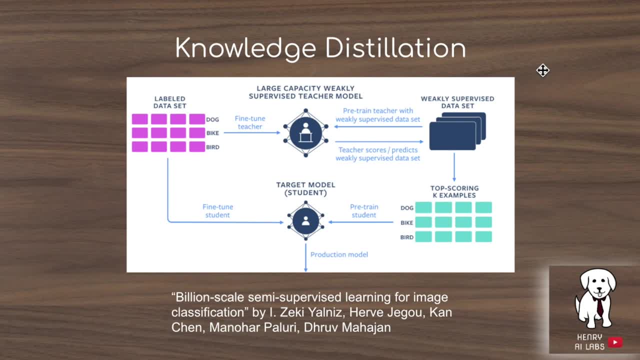 So typically this is what knowledge distillation is used for, but recent research has been looking at knowledge distillation as a way to achieve state-of-the-art accuracy. Another similar study recently from Facebook is this study: Billion Scale: Semi-Supervised Learning for Image Classification. where they use 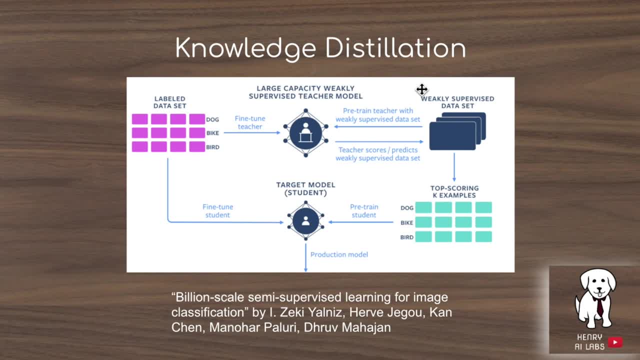 the teacher-student knowledge distillation pipeline in order to make use of weekly supervised datasets, in this case, using weekly supervised Instagram images, where they're labeled by the hashtags that have been provided by the user uploads, and they use this to pre-train the teacher network and they fine-tune. 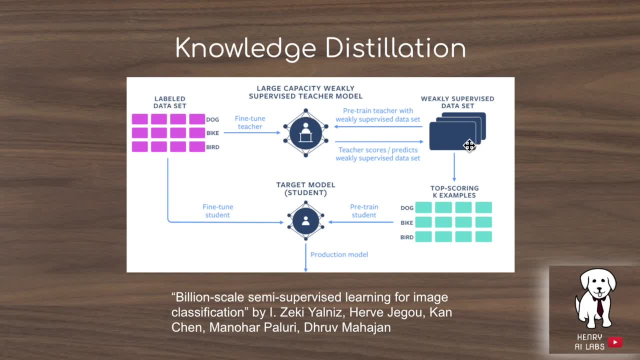 the teacher network and they use this to pre-train the teacher network and they fine-tune the teacher network with the labeled ImageNet dataset. Then they redo this class distribution on the weekly supervised dataset which is used to pre-train the target student and the target student is going to be: 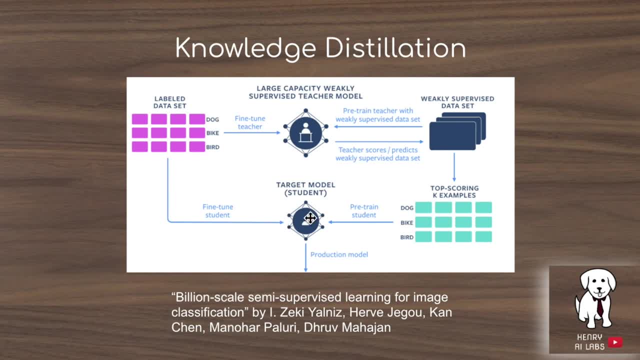 fine-tuned on the original dataset. So this paper from the Google AI Research Lab differs from this in a few ways. One is that it trains on the combined of the fine-tuned and the pseudo-labels from the unlabeled dataset, but in addition, it's going to be an iterative algorithm. So the teacher. 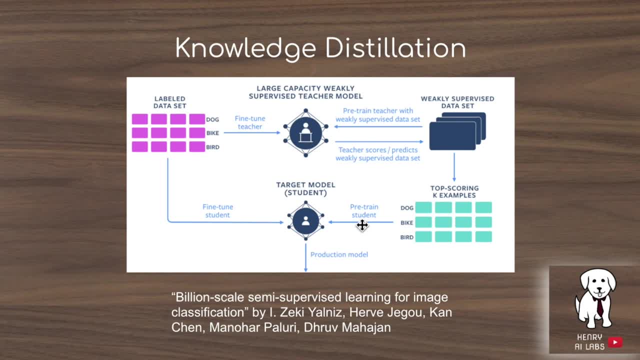 is going to start off as a B7 efficient net and then it's going to scale up to this L0, which is a larger version of the largest model of the EfficientNet, and then it's going to iteratively go from, say, L0 to L1, and then L1 to L2, and then it's going to stop from L2 to L2.. So it's iteratively. 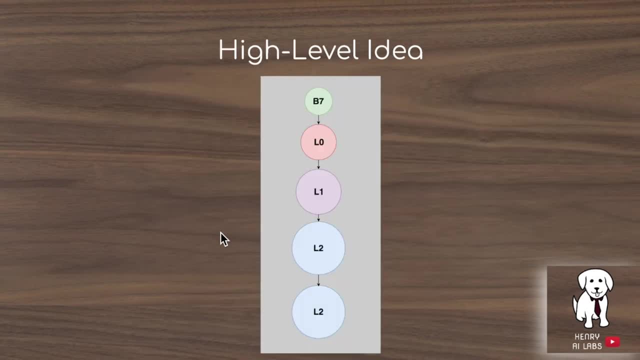 going to be scaling up the size of the student network. This image quickly describes the high-level idea of how they're going to iteratively scale up the student networks in the teacher-to-student knowledge distillation pipeline. So they start with the EfficientNet B7, then they go to the 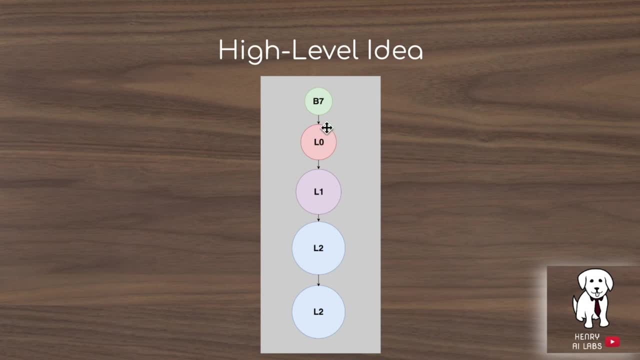 larger capacity. L0 as the student network. that's predicting the pseudo-class labels from the B7 architecture, trained on ImageNet. So then they're going to scale up the size of the student network and do the same thing. Now the student network becomes the teacher training, a higher capacity. 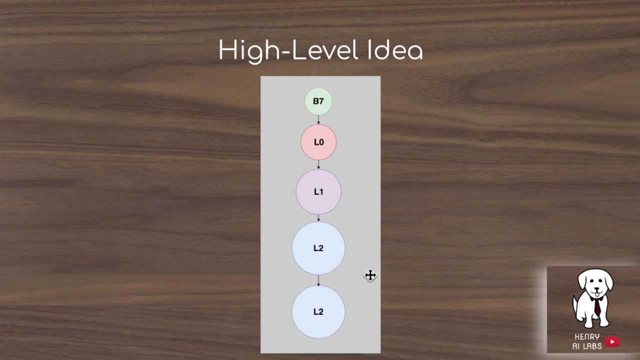 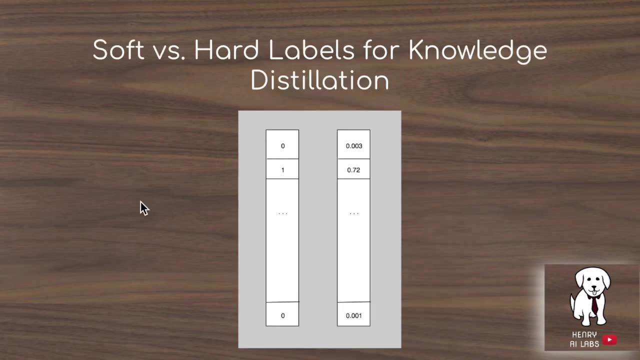 model, and this iterative pipeline continues in this case up until the L2, which is a basically a scaled-up version of EfficientNet. Another quick, interesting characteristic about knowledge distillation is the use of soft versus hard labels, So hard labels would describe this kind of. 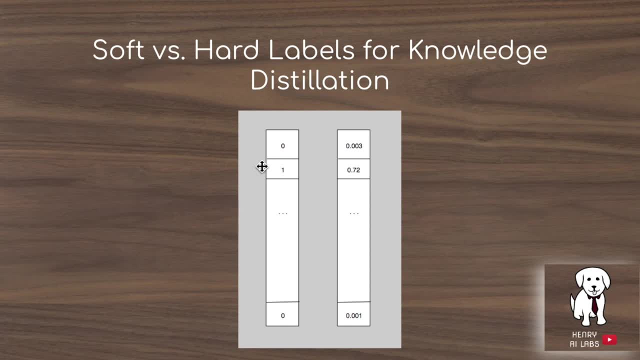 distribution on the left where you have this one denoting the class label, So say this is dog and this is cat and this is, you know, all the other ImageNet classes up to say something like ship. This would be a hard label distribution where you just have one for the class label. 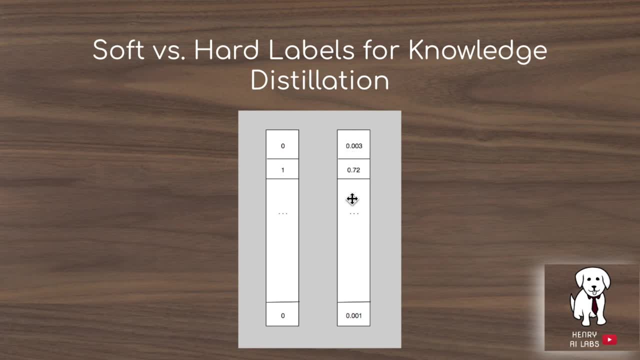 and then zero everywhere else, compared to the soft labels, which is what is used in this knowledge distillation, where you have the outputs from the neural network. So say 0.003% it's a dog and then 0.72% it's the cat, and then you would take the argmax over this distribution to make. 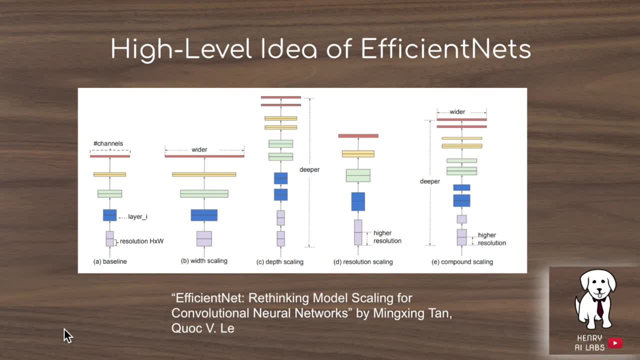 the prediction. Another characteristic of this study that I thought was interesting is the use of this EfficientNet compound scaling technique to scale up the resolution, width and depth of networks in order to have the pipeline from EfficientNet B0,, say, up to B1,, B2, up to B7,. 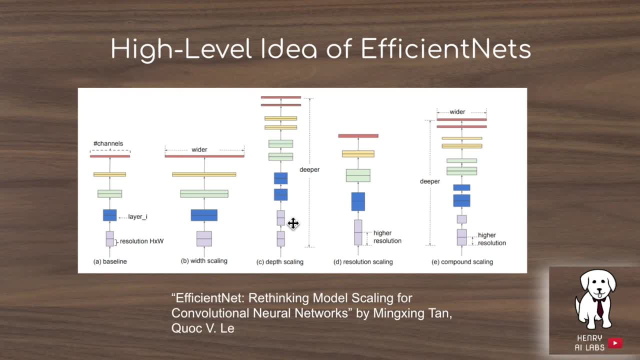 and then up to these L0, L1, L2 networks that are based similarly to the EfficientNet and introduced in this study. So I think it's really interesting how they sort of have this like compositional hierarchy in terms of the complexity, the capacity. So it's definitely interesting to think about this. 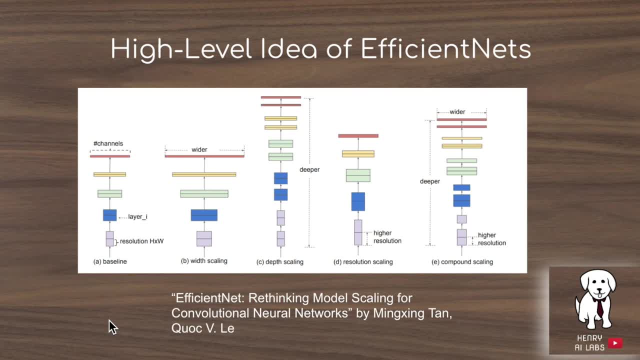 capacity increase from the iterative teacher-student framework in comparison with other networks, like maybe you would have like a ResNet that would go from ResNet 18,, 32,, 50. But the EfficientNet, I think, is more interesting because it has this compound scaling where it's. 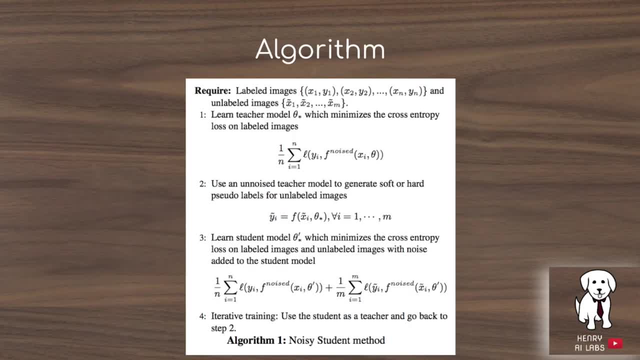 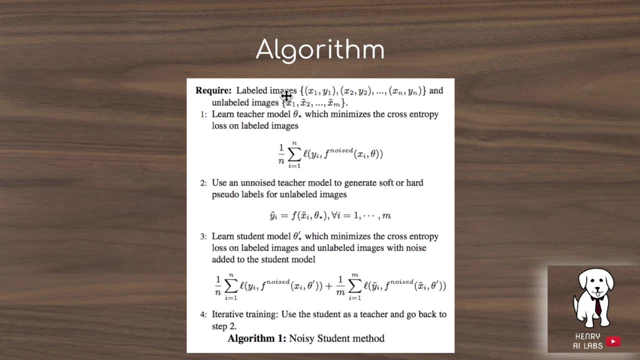 scaling up not just the depth but also the width and then the input resolution. So this is the full algorithm for self-training with noisy student to achieve the ImageNet classification state-of-the-art. So you take in as input the labeled ImageNet dataset. 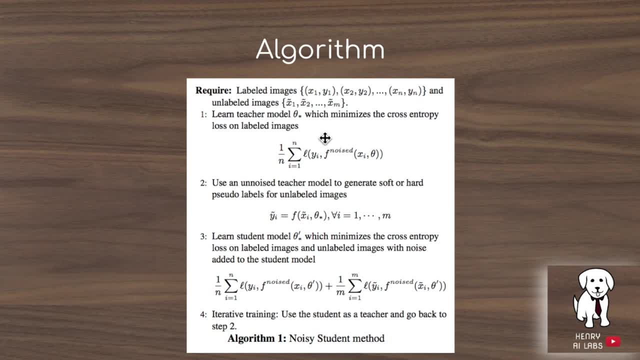 and the unlabeled JFT 300 million dataset. So you start off by training the teacher model using supervised learning, with the cross-entropy loss to classify the ImageNet dataset. So you have noise in the form of data augmentation, like rotations, horizontal flips or you know. 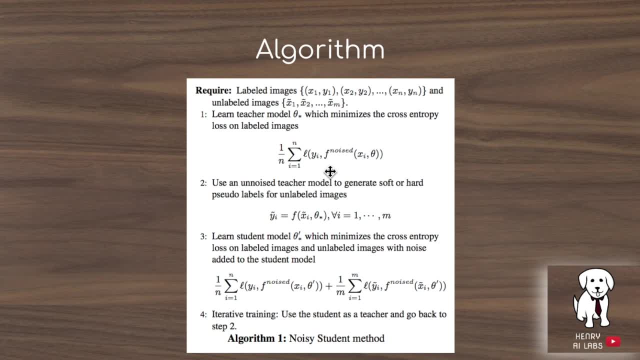 vertical-horizontal shifts of the images, And you also have this kind of noise in the form of dropout, where you randomly drop out the input of certain data. So you have this kind of noise in the form of dropout, where you randomly drop out the input. 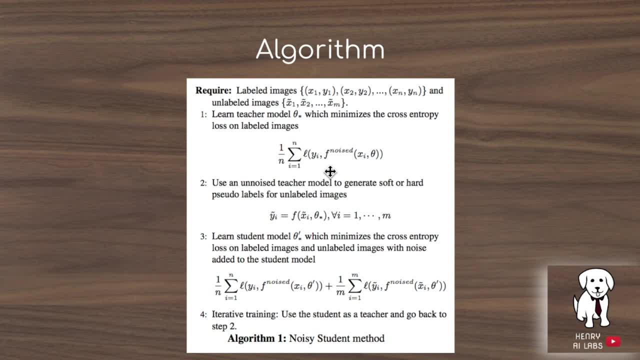 neurons in the forward pass. Then you also have this noise called stochastic depth. So stochastic depth is where you say, take the features at layer 3 and copy them up to layer, say, 8 by using an identity projection, and then you randomly do this to add noise to the network. So once you've 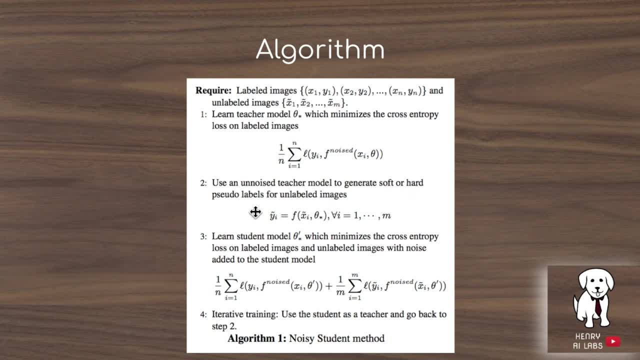 trained this teacher network. then you use the teacher model to generate soft or hard pseudolabels, the difference being soft having things like 0.003, 0.72, compared to hard, which would be 0.1, 0.0.. So this is the difference between these two pseudolabels. In this study, they used the 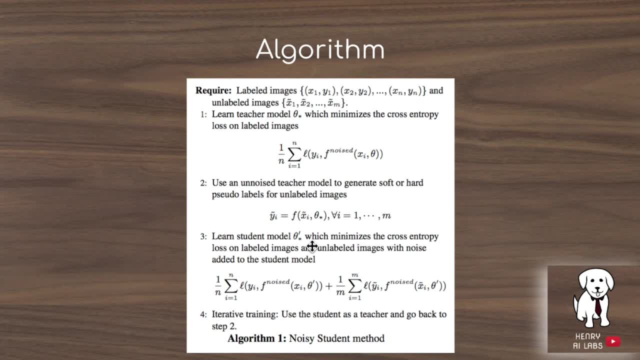 soft labels. So then you use the student model to minimize the loss on the original ImageNet dataset as well as the pseudolabels for the unlabeled JFT 300 million dataset in this kind of loss function, And then you increase the capacity of the student model, the student now. 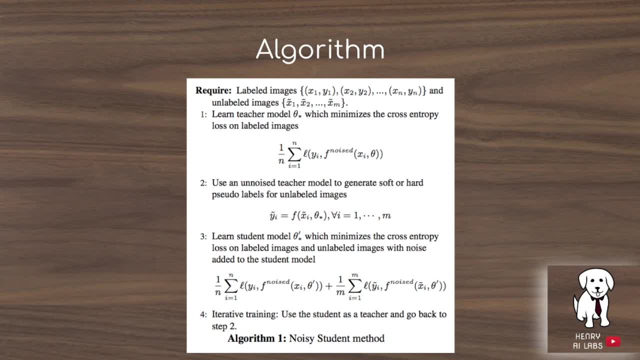 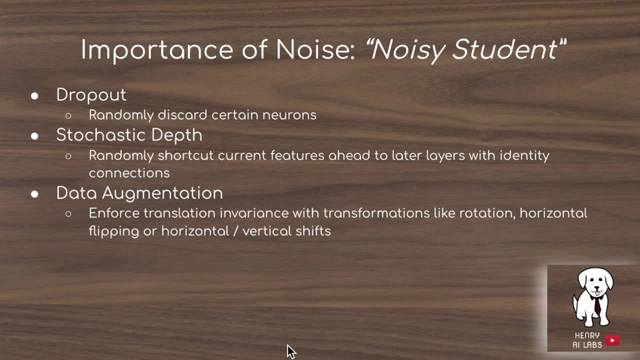 becomes the teacher and then you iteratively repeat this until convergence. So in their study they find that the importance of noise in the noisy student training is really important, even more important than increasing the model capacity up to this L2 capacity. So the three kinds of noise 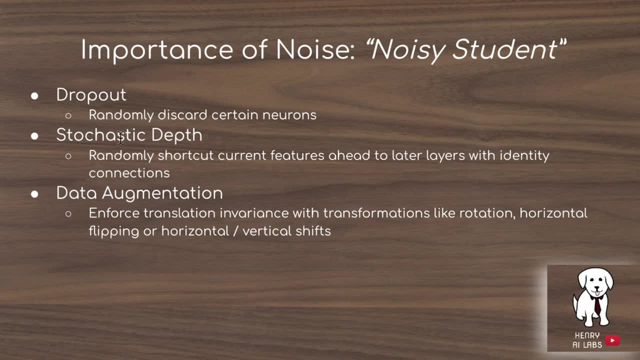 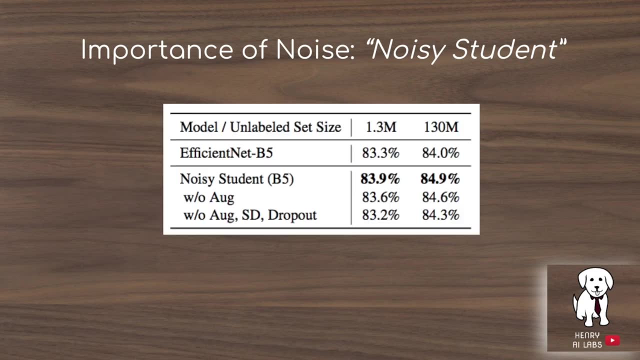 they use are dropout, where they're able to generate noise. and then they're able to generate noise randomly, discarding certain neurons, stochastic depth, randomly, having shortcuts to later layers, and then data augmentation to enforce this translation invariance. So they also have a 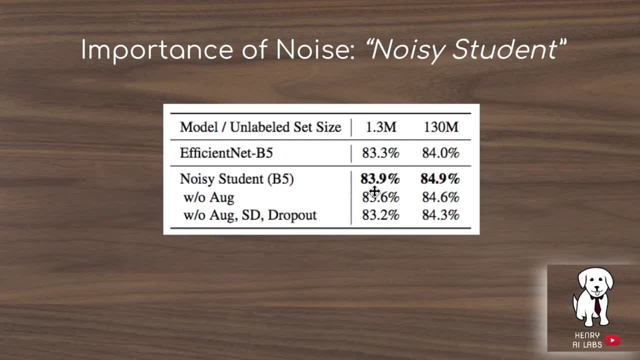 ablation study showing the importance of noise. So you see the difference between when they get the 83.9% using the different data- augmentation, stochastic depth and dropout- compared to when they remove it, having the accuracy drop down to 83.2% and then 84.3% from 84.9%, And this up top. 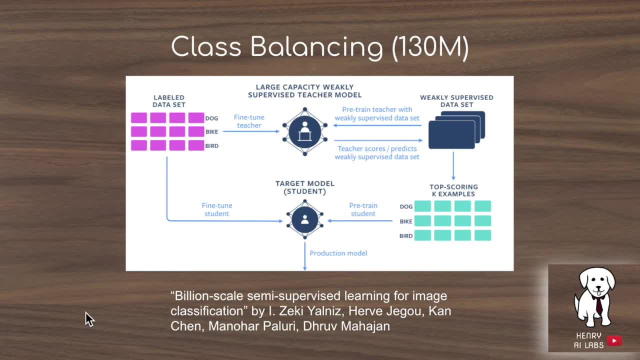 is the effect of the overall dataset. In this study they also use class balancing on the predicted pseudolabels for the unlabeled dataset. So this technique was also used in Facebook's billion-scale semi-supervised learning for image classification. Basically, the idea is that you don't want the student network to be corrupted. 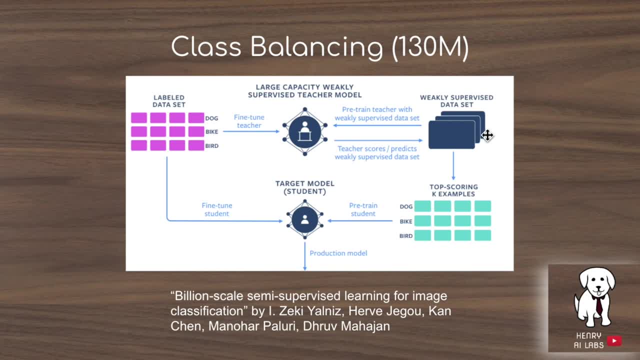 in its dataset with the pseudolabels due to class imbalance. So say, the teacher model has been trained on ImageNet and then it's getting this unlabeled dataset that's out of the distribution of ImageNet and it might predict classes in a certain way. It might not really have an even. 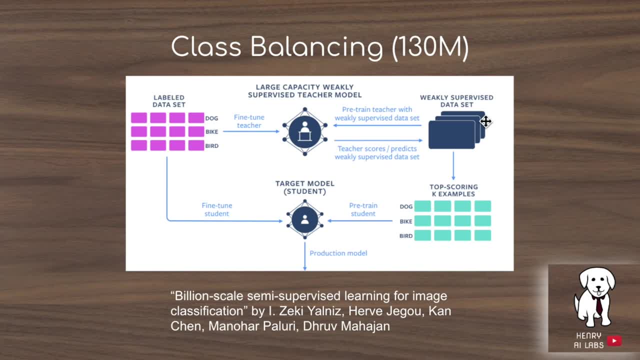 distribution over the 1,000 ImageNet classes. So the way that they handle this is by using the self-training with the noisy student in this paper. They do class and balancing to make sure that they only have 130 million images in the dataset and they do this by doing randomly oversampling. 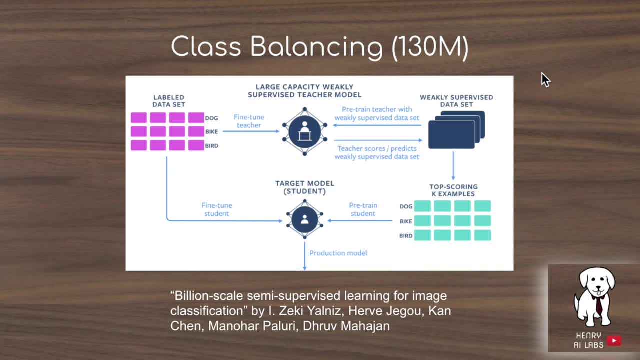 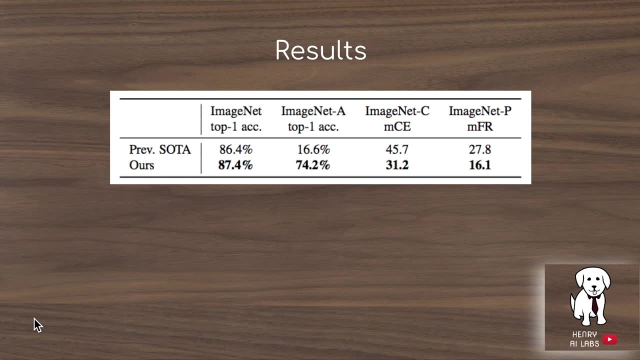 for the classes that don't have enough sample points, and then they only take the top K confidence samples from the classes that have more than the threshold of samples. So these are the results from the study. Some of the interesting results as well are that not only do they achieve the top one, 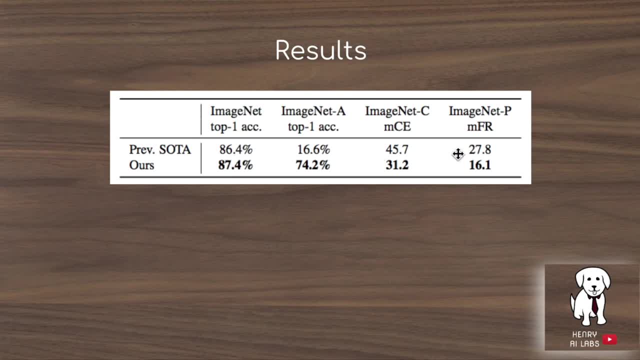 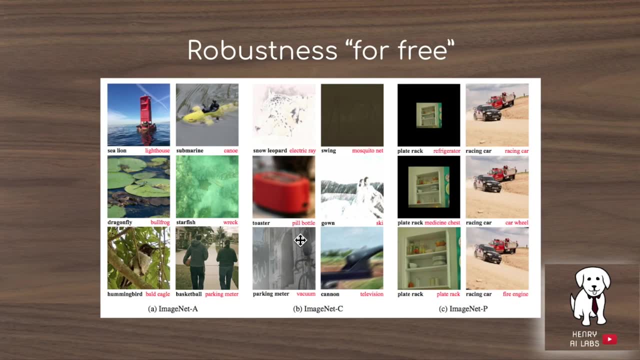 accuracy on ImageNet improvement. but they also have this kind of robustness for free, meaning that they didn't deliberately train for this robustness, So they don't have to do a lot of this on the ImageNet A, ImageNet C and ImageNet P datasets. So these are the kind of datasets. 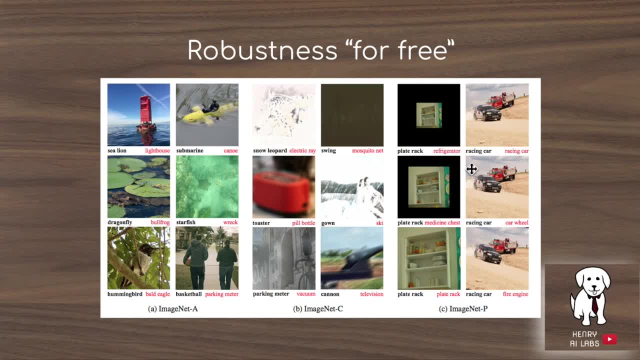 This is ImageNet A, C and P. C and P are basically different kinds of augmentations, different levels of augmentation. You see things like the motion blur and different kinds of augmentations, things like horizontal flipping, and then you see on the A case are examples of hard samples from 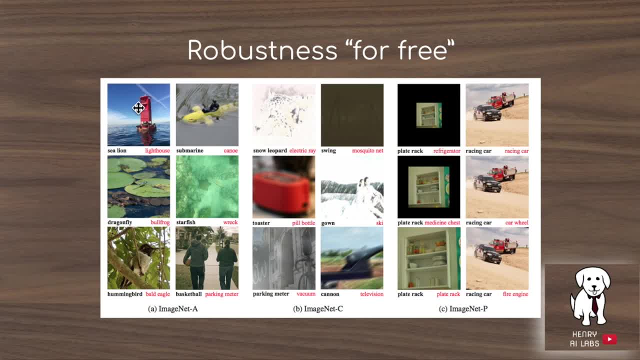 the ImageNet that are tough to classify. So, for example, this image on top: the original classifier classified the buoy as a lighthouse, when it's really supposed to be sea lion. The paper also provides the following charts to show how their new technique has improved over previous models. 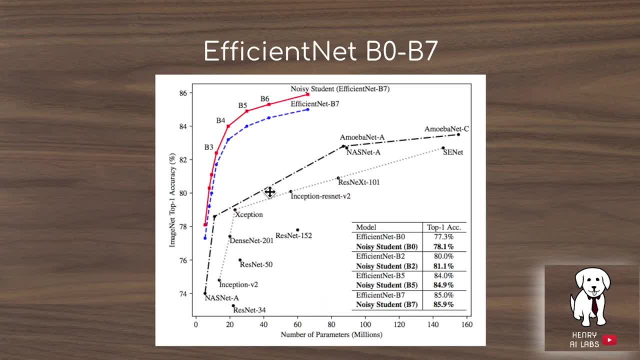 on having this kind of robustness for free. So also in the study they show how this kind of scaling up with the noisy student works on the EfficientNet pipeline from B0, B1, B2, B3, up to B7. Comparing it directly with the original EfficientNet B7, you see the noisy net slightly. 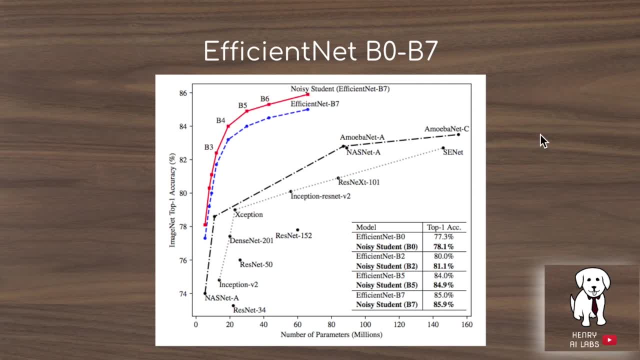 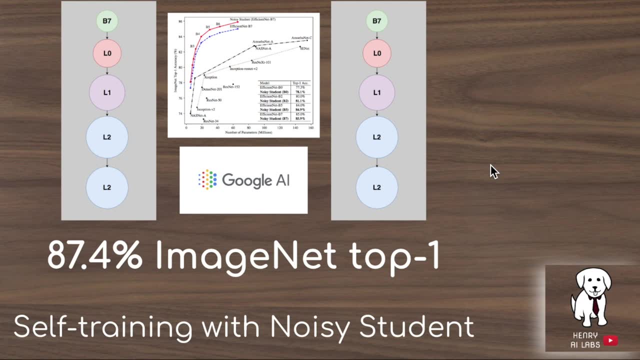 outperforms it and definitely interesting to see this kind of scale compared to the EfficientNet B7. When they have the really large scale, L0,, L1, and L2 networks. Thanks for watching this explanation of self-training with noisy student A new.